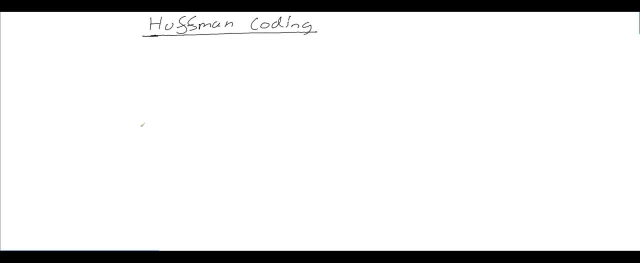 compressing data uses something called a Huffman tree, And I'm going to show you what one of those is with an example. So my example is going to be that I want to compress the text Hello World. Okay, so Hello World. And what we first got to do is we've got to look at the characters in Hello. 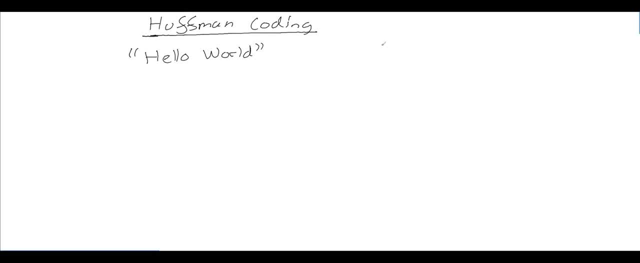 World and see how frequently they occur in a text. So I'm going to do a little table over here. So the first character we've got is L, And I'm doing this in frequency order, So we can see here that L is the most frequent character. 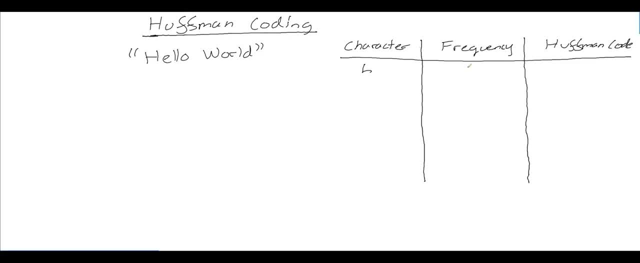 in this text because we've got one, two, three L's. The next most frequent character is O, and that's because we've got two O's in the text And all of the other characters there is just one of, so I'm going to write those in and it doesn't matter which order I put those in my table. 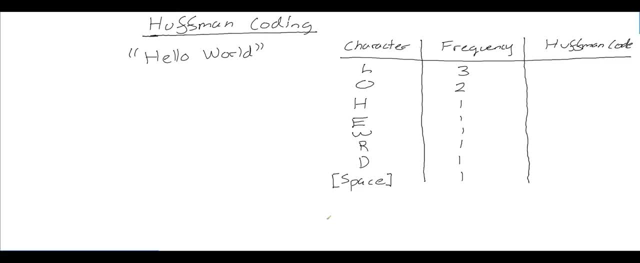 Okay, so those are all the characters which go into making up the text Hello World, And you'll notice here that I've got this space character here And that's because where we've got space in our text, that is stored as a character in memory as well. And 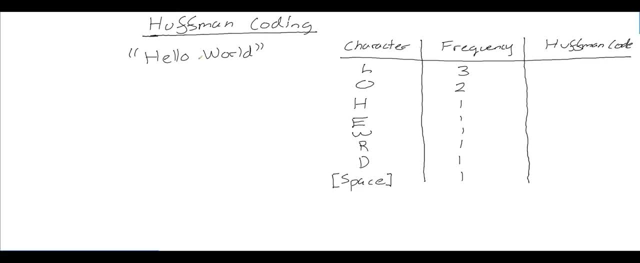 there'll be an ASCII code for that if you were, for example, encoding your text in ASCII. So we've got to include that in our running through of the Huffman coding algorithm as well. So what is the? So to find out what our Huffman code is and which is going to be, in total, take up less bits than 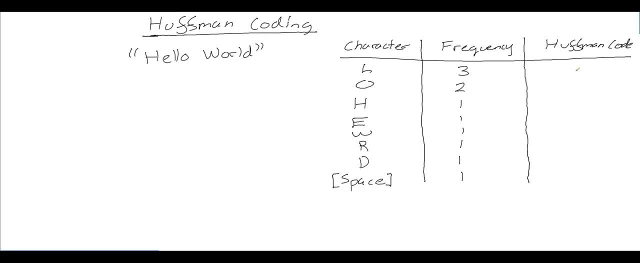 ASCII. I'm going to be comparing it to how much, how many bits, the same text will take up in ASCII. at the end, We've got to construct a Huffman tree, and that will allow us to work out the Huffman code for each character. So how do I do that? Well, what I've got to do is look at each character here. 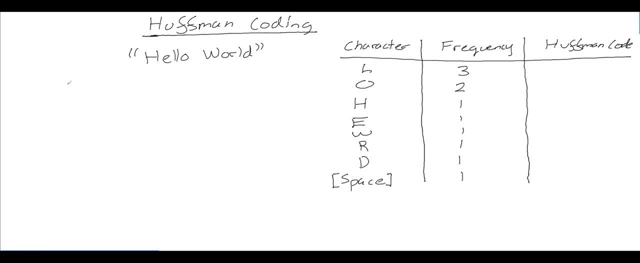 and put them in frequency order, going from lowest at the top to highest at the bottom of a list of nodes, And these are going to be the nodes in our tree. So I'll just do that now. So we're going to abbreviate space to SP, which will save a bit of time. Okay, so those are my 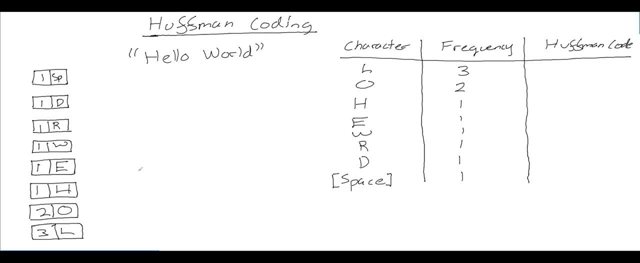 nodes And those are going to form my Huffman tree And you can see of each node I've got a number representing the number of times that character occurs in our text And I've got the actual character in there and I've abbreviated space to SP. So what is the first part of our 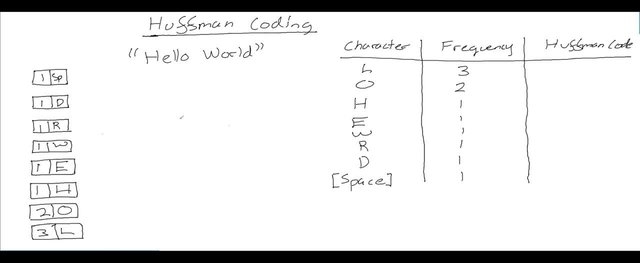 algorithm then. So, first of all, what we've got to do- and we'll put a line down there because that's that's step one of our algorithm there- to create those nodes. And the next step is to take the top two nodes and add the frequency of the characters together and then slot that back. 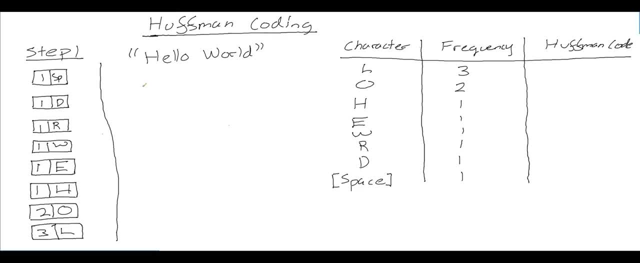 into the list of nodes So that it is still in order. I'm going to show you what I mean by that now. So what I've done is I've taken the top two nodes. So in step one that was space and D. 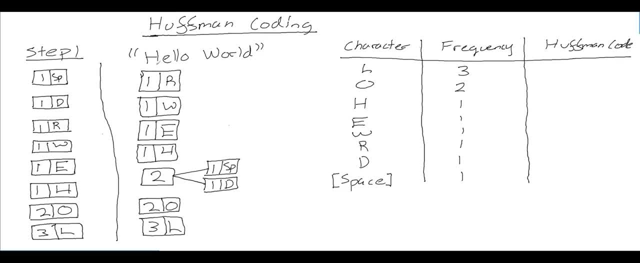 and they are both. they both occur once in our string of text, So I've added the number of occurrences together so I get two. then what I've done is created a new node with just two in it and slotted that new node back into the list of nodes that we've got. 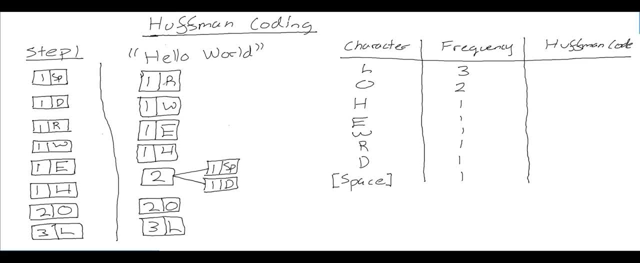 which. so it's sort of it's in order still. So we've got our ones, twos and threes- value, value of occurrences- And then I've taken two lines out here and attach the space and D to the end nodes here So you can start to see that this is how we're going to build up our tree. So we're going. 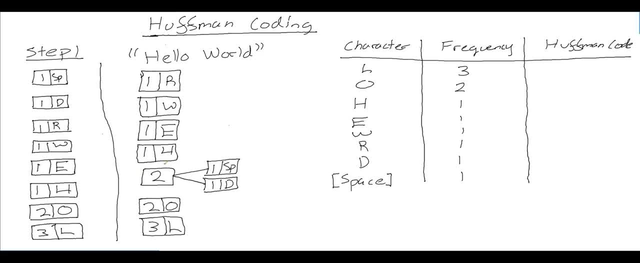 to repeat that process until we've only got one root node and we've got a tree expanding out. So I'm going to show you the steps of how to do that now. Okay, so this is the next step of our room. So you can see what I've done here is done exactly the same as I did from step one to step two here. 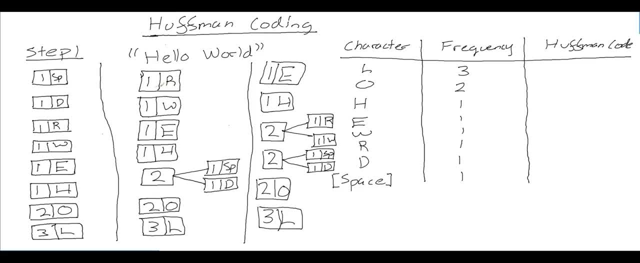 I've taken the top two nodes in this case and I've added a new node to the list of nodes that we've got in place from step two. it was R and W And I've added the frequencies together to get two And I've slotted that back in to the list of nodes so that it runs in order and I've got. 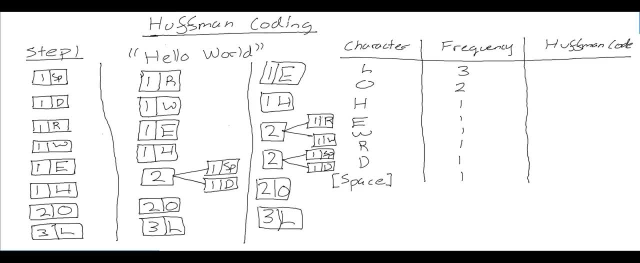 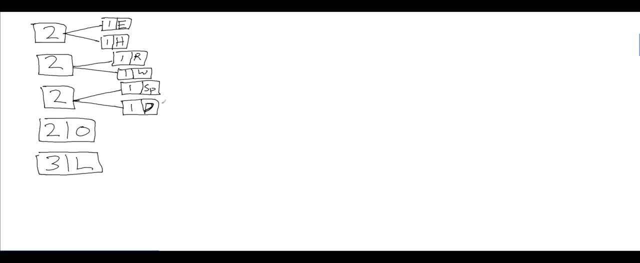 branching off of my new to node. I've got the original nodes that I made this to node out of in terms of the frequencies, And we then got to repeat that again more for this E and H. Okay, so this is the next step of our algorithm. you can see, I've done the 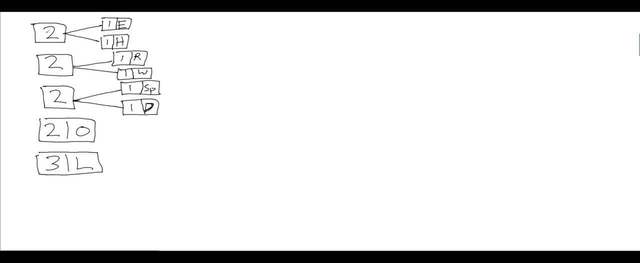 same thing with E and H. I've got a new node, which is two, and I've put it in to the correct place in the list. So we've got 22223 now as our list of nodes And branching off of these. 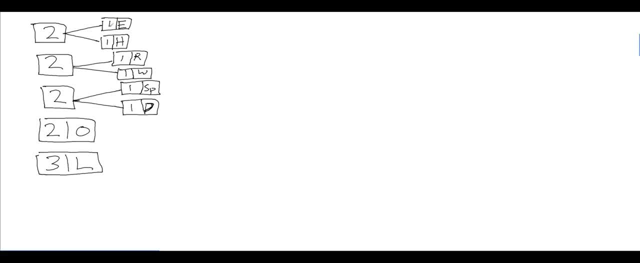 we've got the original nodes that we had in the list, which have a frequency of one. So this is how we start to build: we've got the original nodes that we had in the list, which have a frequency of one, And in the next step, what we're going to do is combine these two top nodes to create one with. 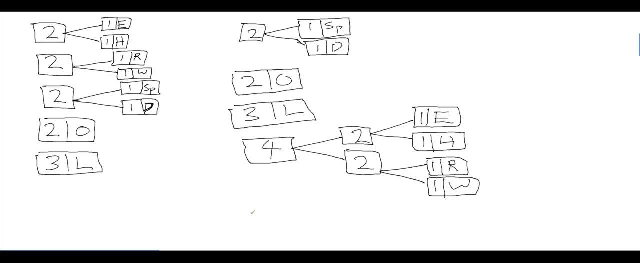 four And I'll show you what that looks like in a minute So you can see again. I'm just repeating that process. I'm adding the frequencies of the top two nodes and I get four as my frequency if I add these two frequencies together, And then I'm just constructing a tree from those two nodes. 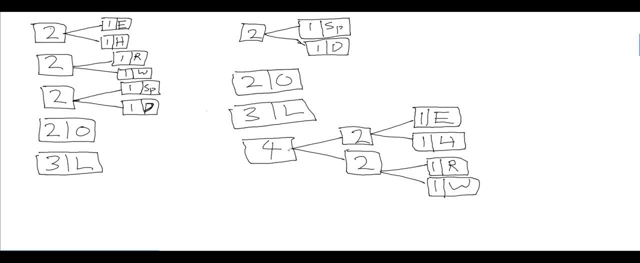 there. So I'm branching off the nodes and then I'm just adding the frequencies of the top two nodes And then I'm just constructing a tree from those two nodes there. So I'm branching off the node with a frequency of four and having these two parts of parts of the tree branching off of. 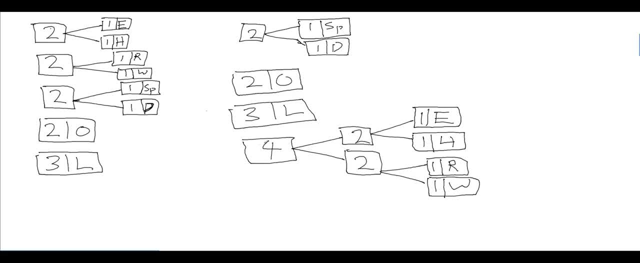 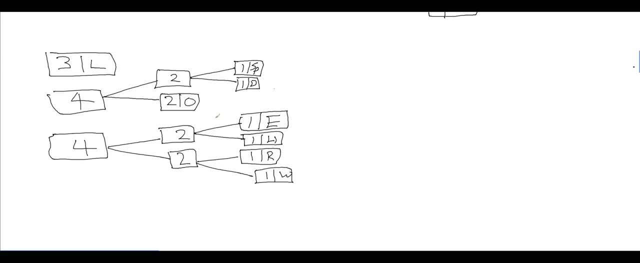 there. So I could continue to do this with these top two nodes here, So I'll get another four. Okay, so this is what my what the algorithm looks like after the next step. So what I've done is I've combined these two, the node with O in, so there's two occurrences of O. 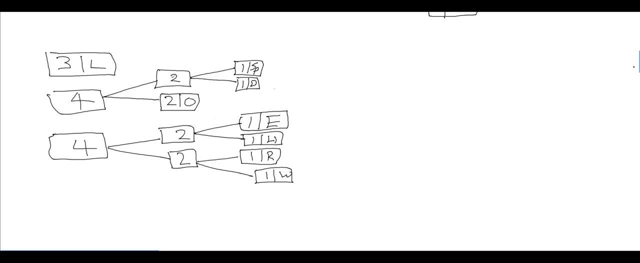 so there's a node of two and O in and this part, this node with a frequency of two, here to get a another node with a frequency of four. put that into the list so that the list is still in order. So we've got a node of three and our other node with four, and it's in numerical order. 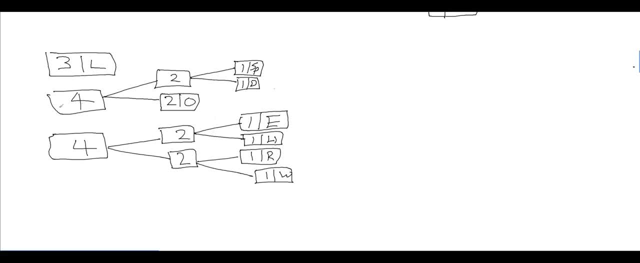 still. And then what I do next is repeat this and take the top two nodes, so four and three, add them together, And then I'm going to get set a node with seven. Okay, so that's the next step. If you look here, I've got my node with a frequency of seven, which is made up of this: 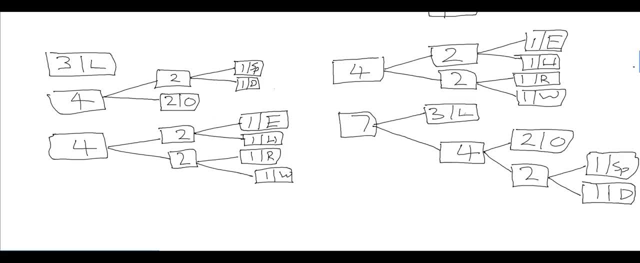 node with a frequency of three, which is representing the character L in our text, and this node of frequency four, which is representing these two nodes, and so on, And we've got the almost our complete Huffman tree. we just need to combine these two. 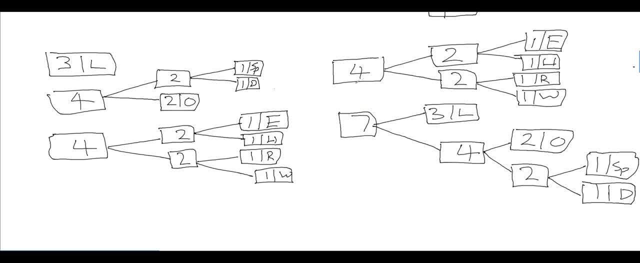 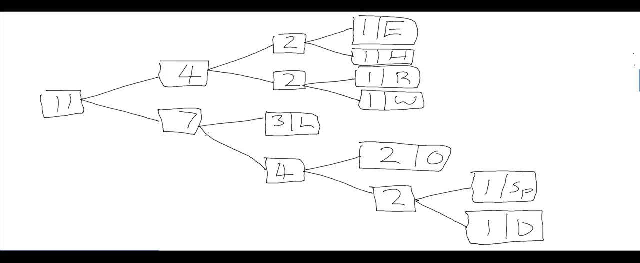 nodes to get a single root node, and if I combine these two nodes, I'm going to get a node with a frequency of 11.. Okay, so this is our final complete Huffman tree, but it's not quite finished yet, because what we've got to do is in order to create a binary code to represent our characters. 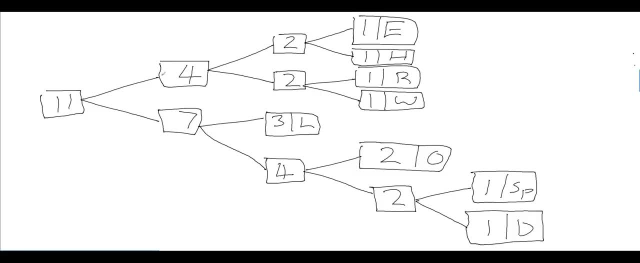 what we've got to do is label each branch going upwards as one and each branch going downwards as zero. What this allows us to do is it allows us to create a code to represent each of the characters, and I'm going to do that here now, and the way I'm going to do that is, for example, if I 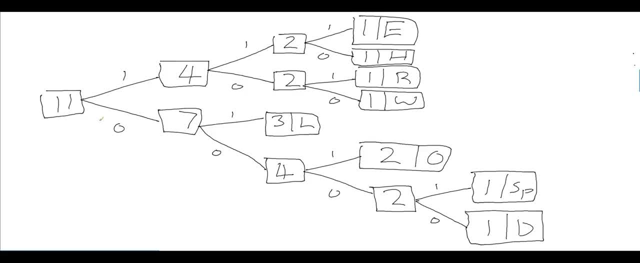 wanted to find out what the Huffman code for the character L was. I would go along the, I would trace along the branches of the tree. so go along here and that's a zero, and along here and that's a one until I get to the node with the character L in. So the Huffman code. 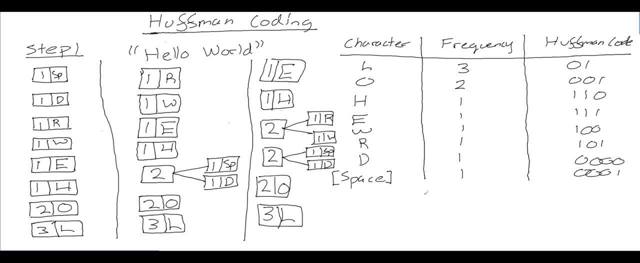 for the character L is going to be zero one. Okay, so from the Huffman tree that I showed you a minute ago and I showed you how to construct, I've come up with this Huffman code, and if I was to represent the text hello world, I would go to the Huffman code and I would go to the Huffman code and I would. 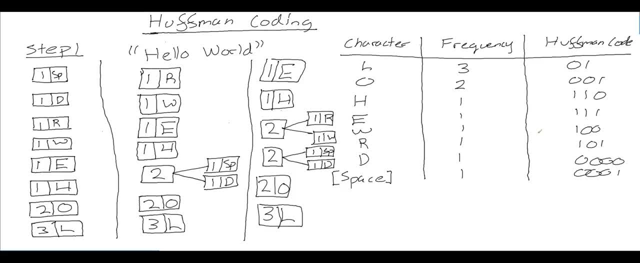 say hello world in 7-bit ASCII, I would need 7 bits to represent each character and there's 11 characters, so I would do 7 times 11 to work out there would be 77 bits to represent hello world. but with my Huffman code what I could do is I can add up how many occurrences and how many bits. 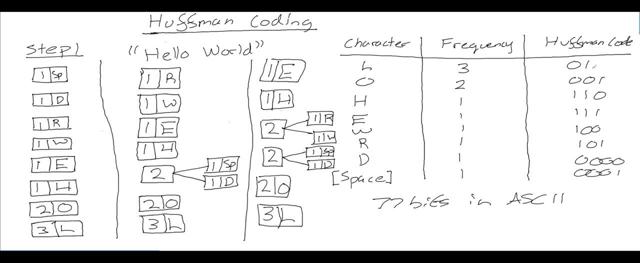 each character would be in my Huffman code. so, for example, if I wanted to work out how many bits the L would be, I would go to the Huffman code and I would go to the Huffman code and I would say: hello world. in 7-bit ASCII I would do 7 times 11 to represent the human Huffman code. 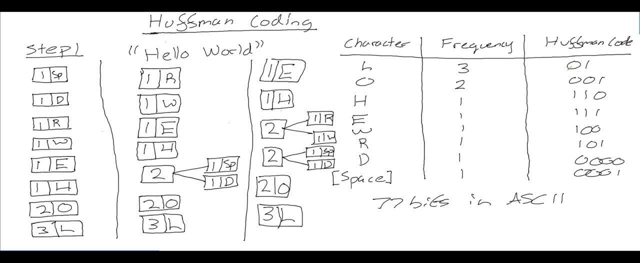 and I would say: hello world. in 7-bit ASCII, if, as seen in the panel, is the first character, theq feature would be Huffman code. so we would do 7 times 11 to represent the human Huffman code. and so that's how we would substitute the letters up. so that's able to какой curse? 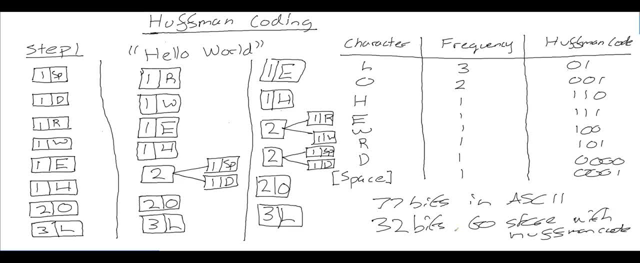 or sum up the number of bits that does not match the key figures like same and you hear, required. but that's ignoring the space required to store the Huffman tree, because you would need to store the Huffman tree in order to decode a Huffman code, to decode something in Huffman code. 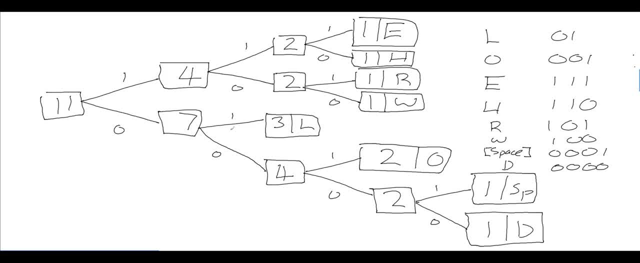 let's have a look at back at our Huffman tree. so for decoding, looking at our Huffman tree, if we want to decode an L, we would go. we would look at the Huffman code, starting at the root node, see that it starts with a zero. so we go down the the branch of the tree with a zero. 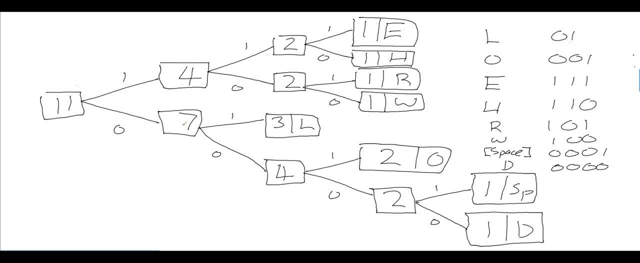 see that the next, the next bit, is a one. so we go up the branch of the tree with a one and we come to the node with no further branches and we see that it's an L. so we D. and that's how you decode Huffman code. you simply traverse the tree using the code that you.